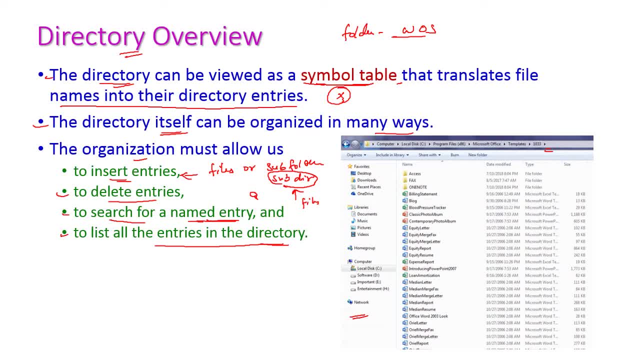 And this is taken from Windows operating system. Okay, Here this is directory. See, from the C disk we are having program files. From this we are having office. So this is subdirectory of this particular one. Okay, From office we are having the template is subdirectory, and 1033 is another subdirectory, So in this 1033, we are having this much files, Right, So here also these two, these three are directories, And 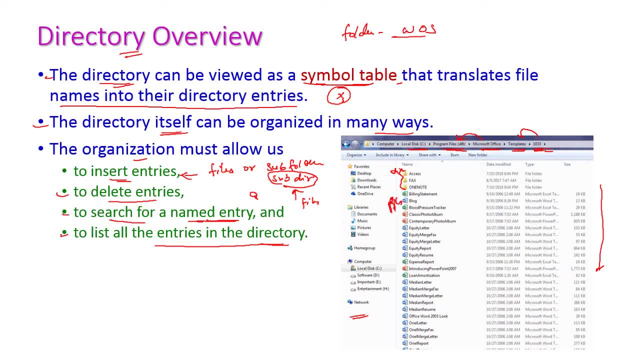 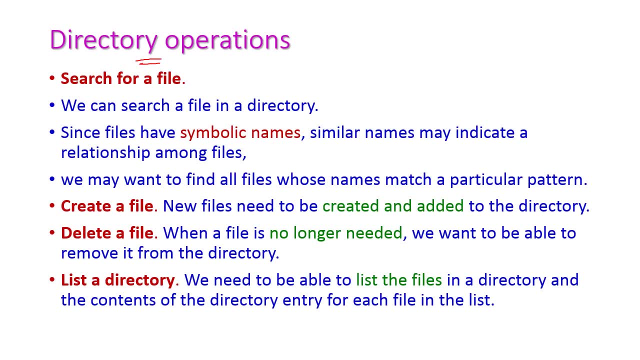 all the others are files, The directory operations. Here. basically, we are having four operations. First one is search for a file, create a file, delete a file and list a directory Right. First let us see the search for a file. We can easily search a particular file in the directory And the file is having symbolic name. That means all the file is having a unique name. 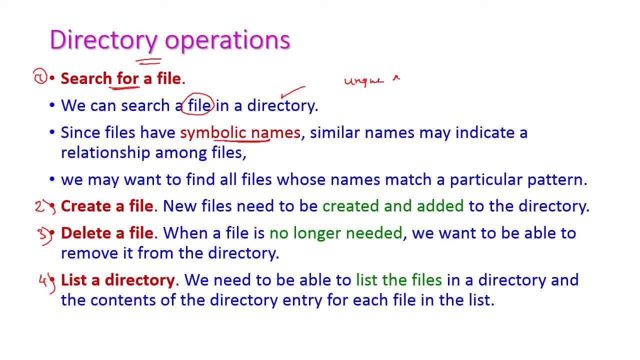 Unique name. Okay Now, the similar names may indicate the relationship among files. So if the files are related to each other, then the similar names may be given for all the files. Hence we may want to find all such files. that is also possible in the search of a file Right. And next one is creating a file, Creating a file used to create and added into that directory. 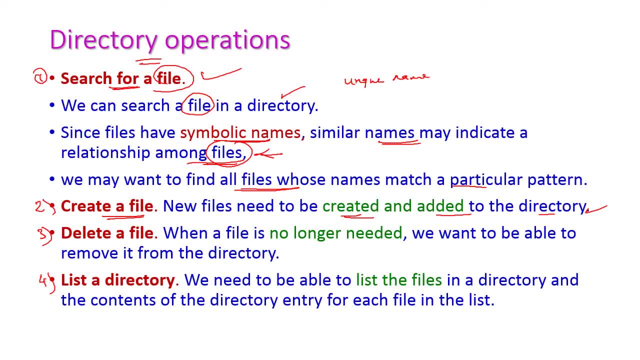 directory. okay, we can easily create a new file and that will be added into the directory and delete a file. if we don't want to need a particular file, then we can easily remove that file from this directory. right, that is, delete a file and next one list a directory. okay, so if we list the directory, 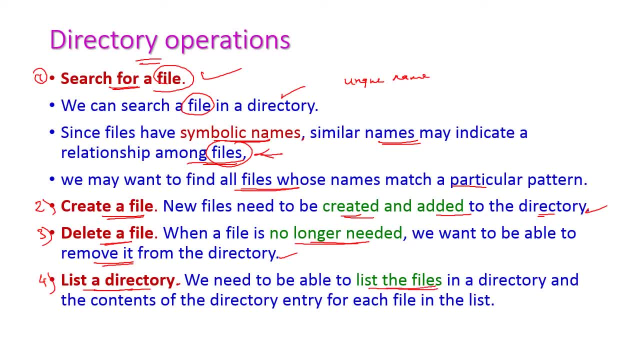 that will list the files which are available in the directory, as well, as the sub directory will also be listed. okay, this is list a directory. so what are the operations here? search for a file, create a file, delete a file and list a directory. the other important operation is rename the file. 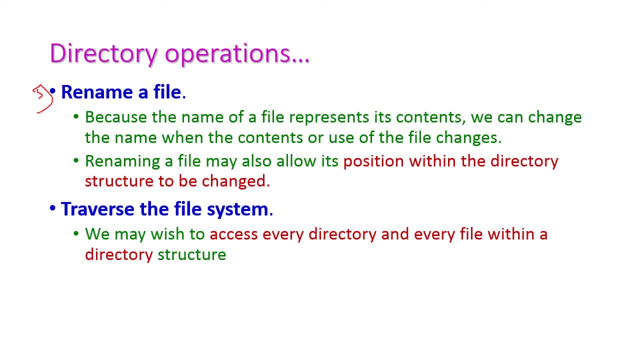 this is the fifth one, because the file name represent its content. okay, based on the content only we can give name for a file. okay, suppose, if the name can be, if the purpose can be changed, then immediately we can give name for a file, and if the purpose can be changed, then immediately. 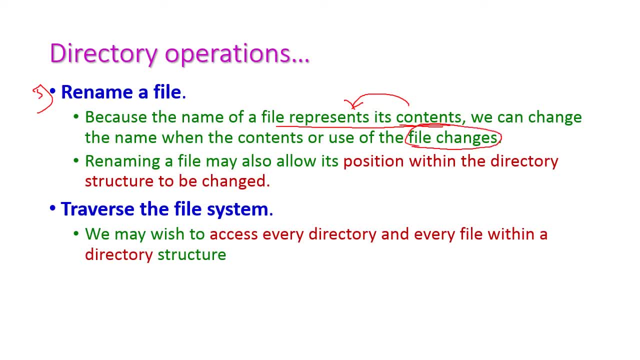 we have to change the file name also. okay, that is allowed by the directory operations. okay, suppose if we rename a file, then the position within the directory structure to be changed, because all the files will be arranged in alphabetical order. suppose if we change any of the file name, the order will be changed. okay, and next operation is traverse the. 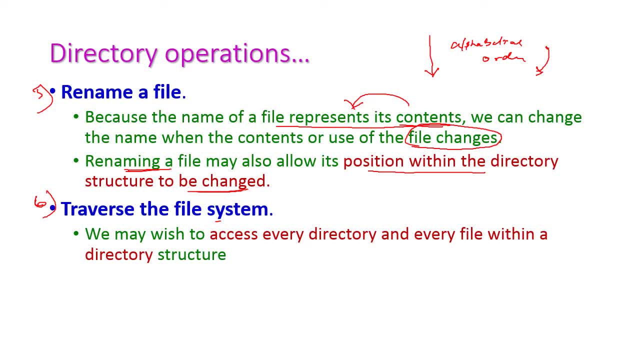 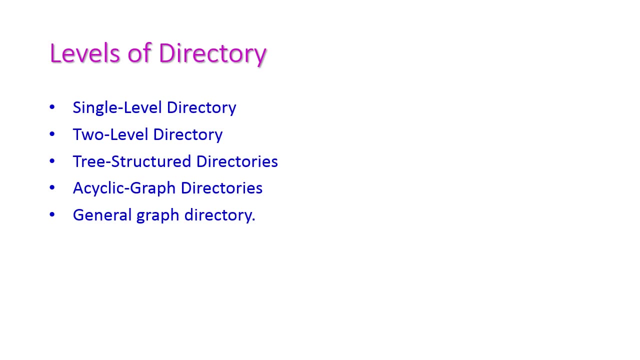 file system. that means if we wish to access every directory and every file within the directory structure, that is possible by using the traverse file system. and next let us see that levels of directory. the first one is single level directory, two level directory, tree structure directory, acyclic graph directory and general graph directory. let us see all those things one by one. first, the 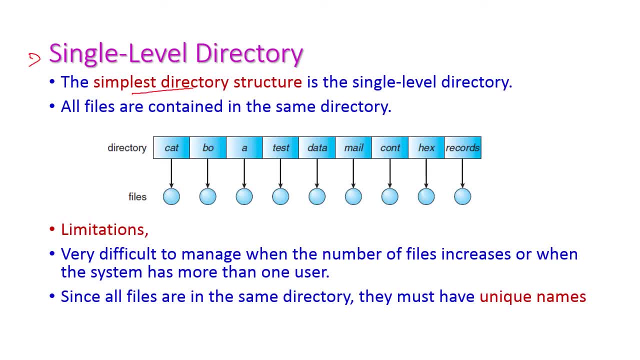 the single level directory. this is a very simple directory structure, very straight forward, because all the files z tycker inge the same directory. okay, we are having only one directory. in this directory, all the files will be stored. right now let us see the limitations of single. 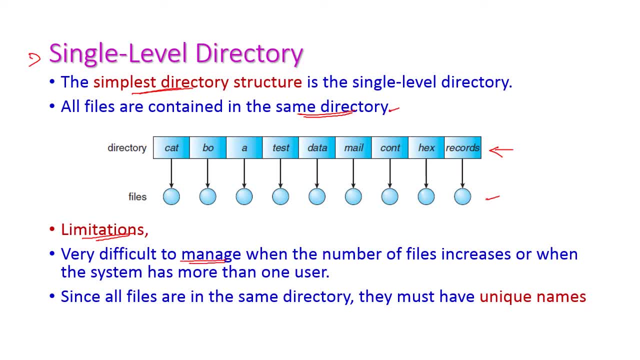 level directory, and this is very difficult to manage when the number of files increase or when the system has more than one users. okay, if the number of files increased, then by the use of single levelaan our files, AS like noted now, and even if the number of files there may be in different direction. history is there are more than this. only the gosp Ut soldiers tail nucleagh. we keep the focus. Duc de Dur technik. this is still vertical, correct, and I will erase the gene code in this case. between this is right by the other operation. we will use the tycker variable. 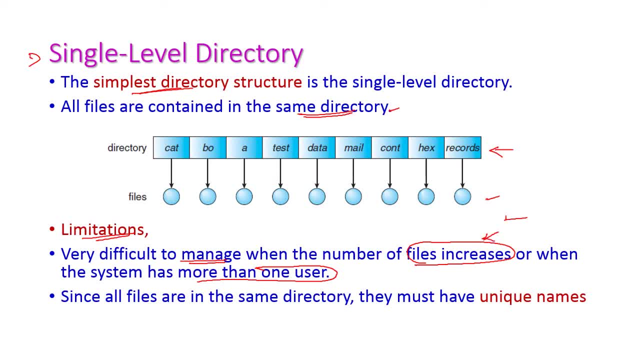 of files increased, then all the files will be loaded in one single directory. then this is very difficult to manage all those files and if more than one user added to that directory then we have to give unique name for all the files and this is highly impossible for all the users can give the unique name. 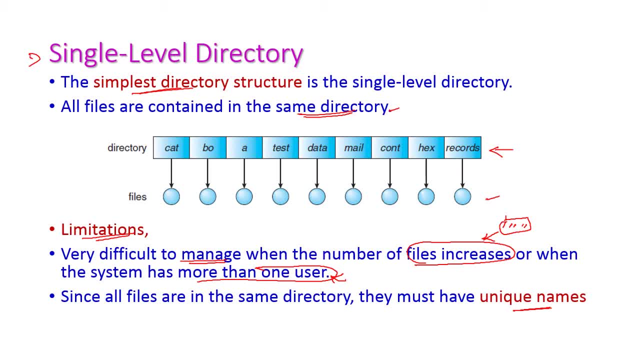 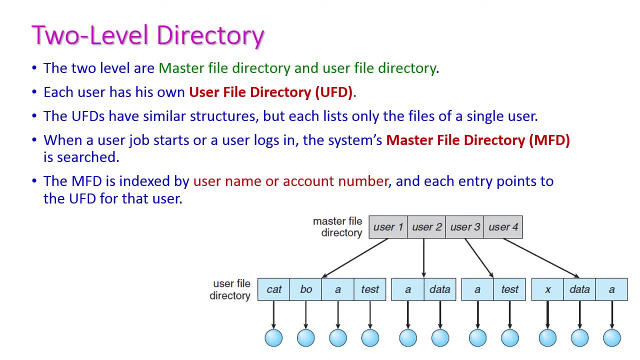 okay. hence the single level directory is very difficult to manage two level directories here. there are two levels of directory. first one is master file directory and second one is user file directory. okay, this is the master file directory- a MFD, and this is user file directory. you have UFD, okay, when come to 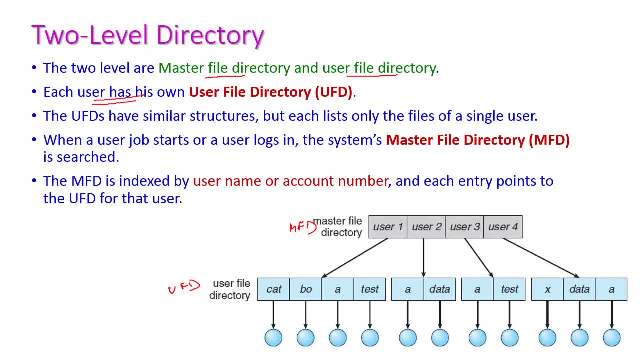 user file directory. each user has its own user file directory and the directory structure is similar. okay, but this directory is only belongs to this particular user. okay, that is, each user has its own separate directory. when come to user job starts, the user logins. okay, user have to. 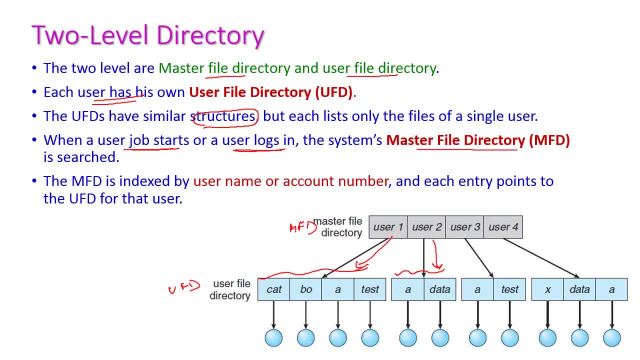 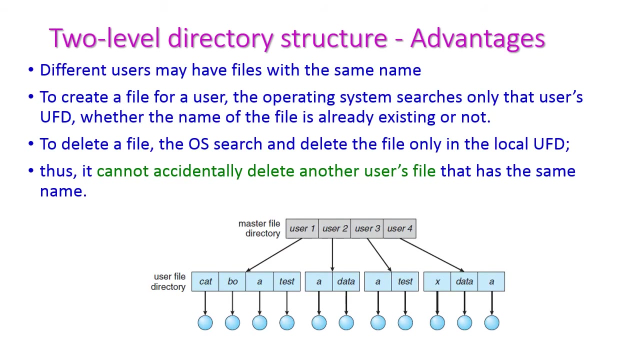 log in, then the system's master file directory is searched. okay, when the user log into the system, then the the system will search the master file directory and find the corresponding user, and the user can access only this particular directory. this is the two-level directory. next let us see the advantage of two-level directory structure. 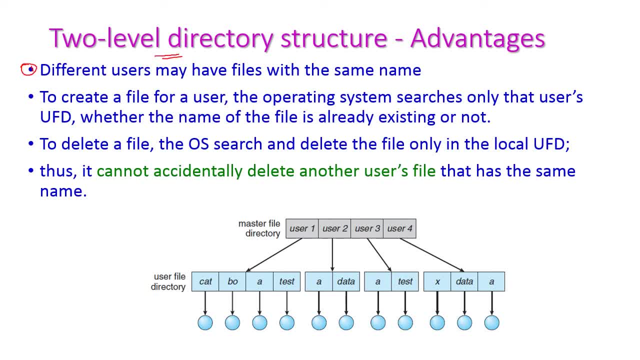 ah, the very big advantage is different users may have the files with same name. okay, this is very big advantage. here we are having four users and just see all the users are having the file. a that means the same named file can be created by all the users. 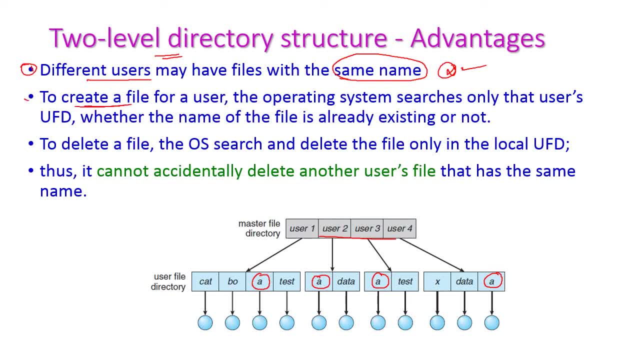 and then we are having a directory, the targeting nodes forusive. all other users are having the Suppose. if you want to create a file for a particular user, then the operating system will search only this particular user's directory. If the file is already existing, we cannot create Suppose. I want to create a file B, then the OS will search only this particular user's directory, whether the file B is already existing or not. 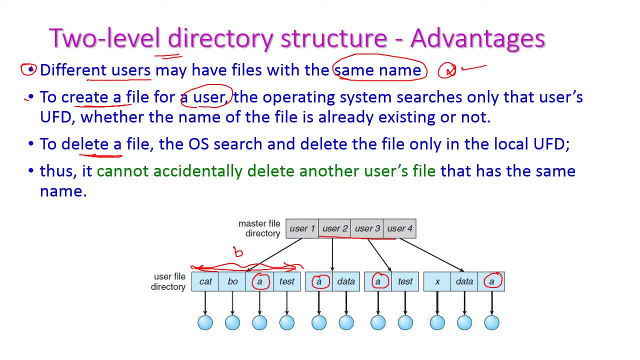 When come to deleting a file, the OS will search only this particular directory to search the file for delete. Hence, suppose I want to delete a file A this particular directory and it cannot accidentally delete other user's file and the other user's file A will be available. 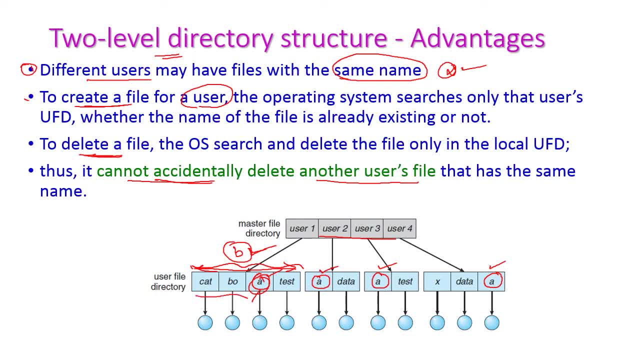 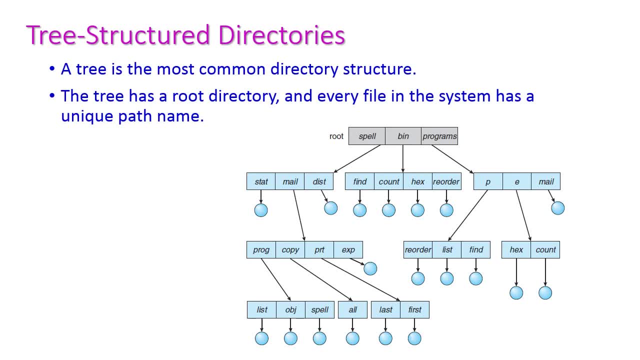 The OS will search only this particular user's directory for creating a file. This is the most common directory structure nowadays we are using and it has a root directory and every file in the system has unique path name. Here this is the root directory. The root directory has its own files, as well as sub-directories and a set of files. 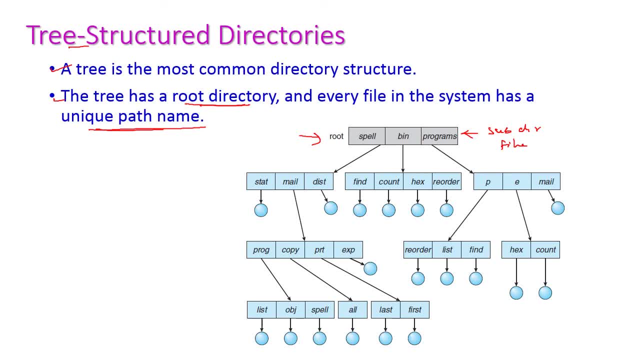 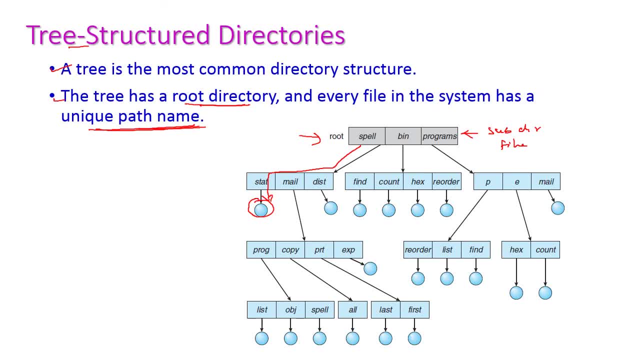 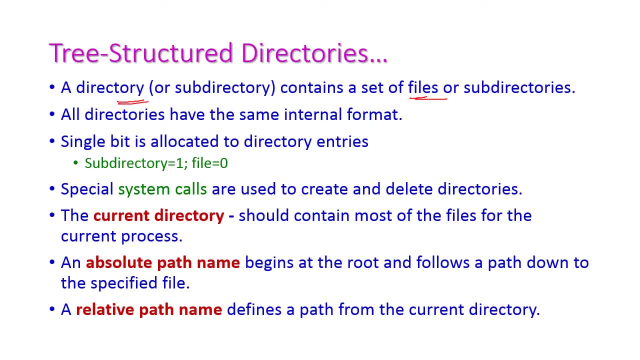 This is the path of this particular file In this tree structure directories: a directory which contains a files or sub-directories, and all directories have same internal format. That is, the format of all directories should be same and the directory should contains a sub-directory or files, and a single bit is allocated to directory entries. 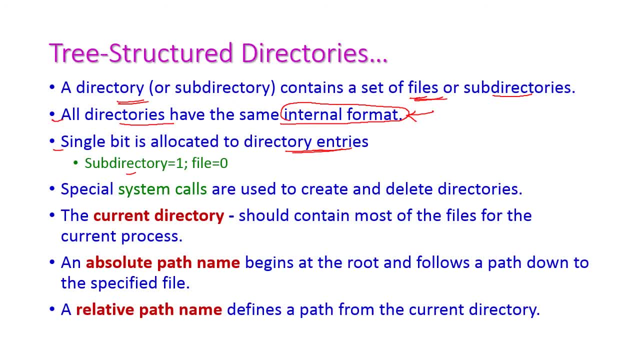 So the directory contains both sub-directory and files, isn't it? For sub-directory the 1 is allocated and for file, 0 is allocated. If it is 0, then we can identify this is file. If the entity is 1,, then this is sub-directory. 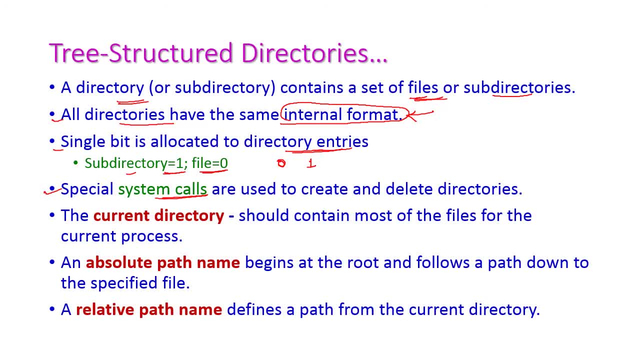 And a special system calls which are used to create and delete directories right And the current directory. current directory means it should contains most of the files which is currently required for the current process, And absolute path name means the path begins root and follows the path down to specific file. 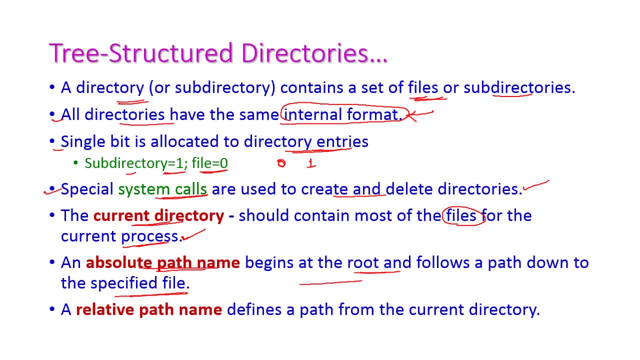 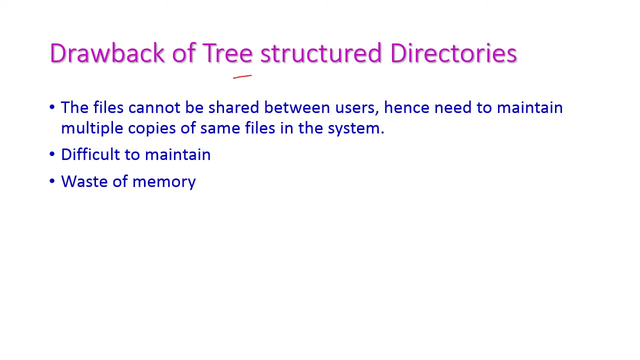 That is the path name starts from root to the specific file, And relative path means the path starts from current directory, current directory, to that file. okay, That is called as relative path. The drawback of tree structure directory: here the files cannot be shared between the user. 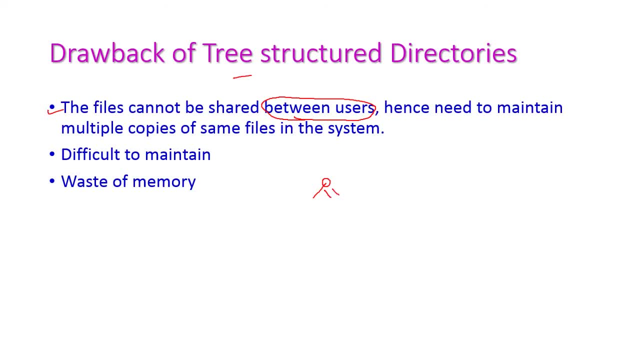 Suppose if the same file wanted by all the user. this is not possible to share the single file for all the users, So we need to maintain a separate copy of the same file for all the user right. Hence it is very difficult to maintain. 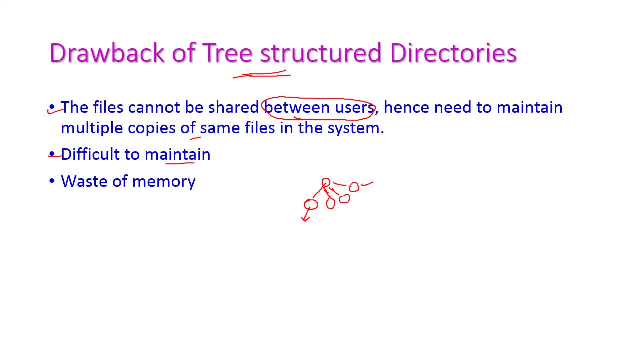 If there is any changes in this particular directory or this particular file, this cannot be reflected in all the other files in different folders, isn't it? So it is very difficult to maintain And the same copy will be replicated in all the other directories. 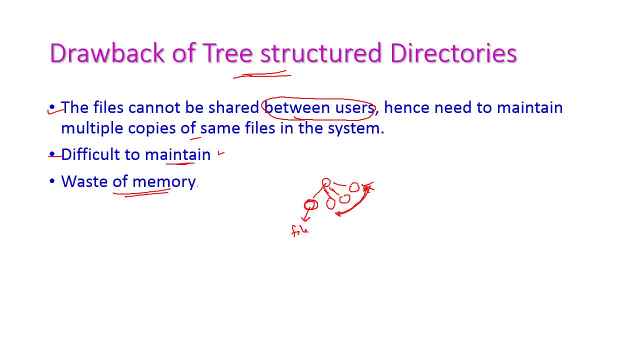 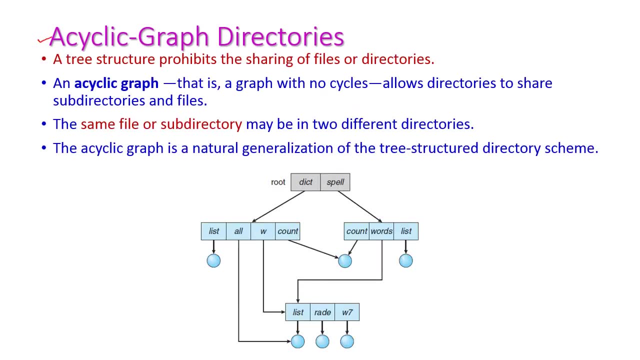 Hence it occupies more memory, So waste of memory. Acyclic graph directories. So this directory is introduced to overcome the drawback of tree structure directory, because in this the sharing of files or directories are highly impossible. okay Now, acyclic graph means a graph with no cycles. 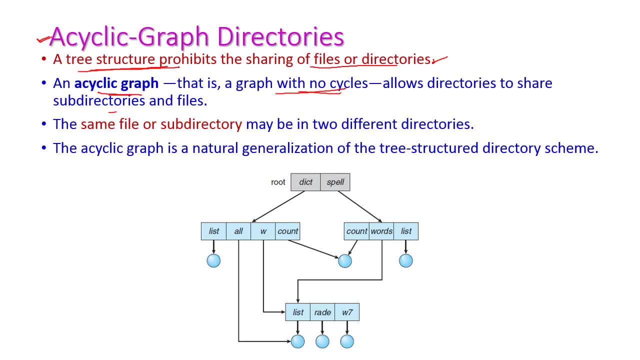 That means this allows the directory to share the subdirectories and files. See When Come here. For example, this is file A. The file A can be shared by both the directories. Okay, Those are from different users, Okay. 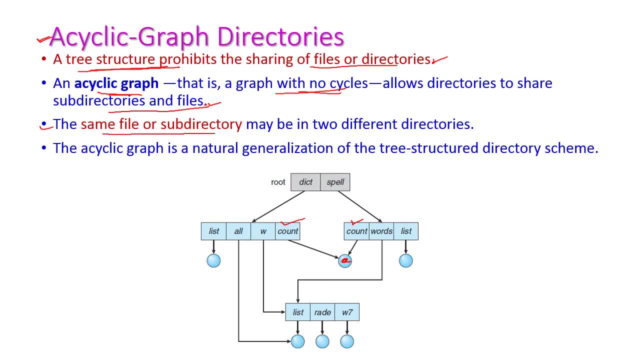 Now the same file or subdirectory may be available in two different directories. Okay, Here the acyclic graph is natural generalization of tree structured directory scheme. Okay, All the other schemes are just like same as tree structure, Except This particular sharing. 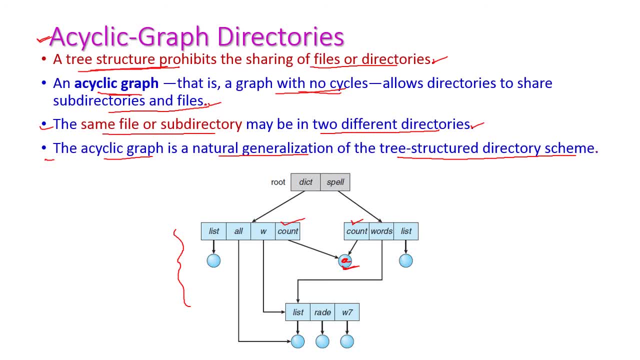 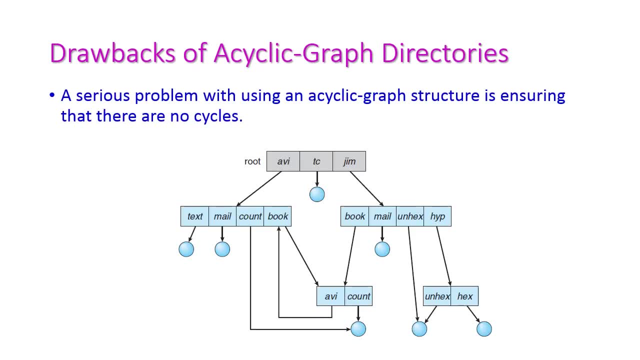 Okay, If we do sharing, then the memory will be saved and the maintenance will also be very much easy. The drawback of acyclic graph directory means if there is any cycle occurs- See in this diagram- this is a cycle. If there is any cycle occurs, then the user will face a series of problem. 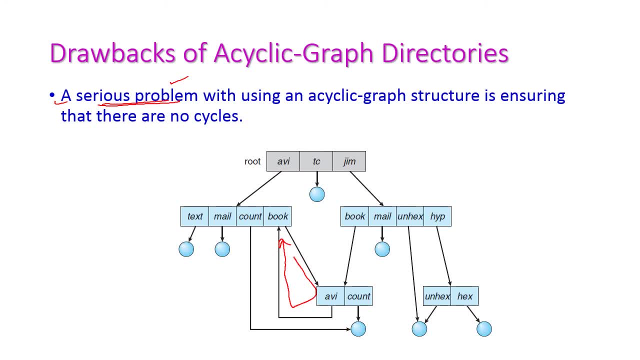 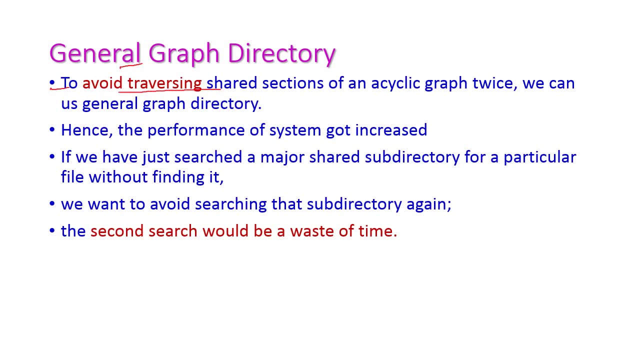 Okay, This is very big Drawback. Drawback of acyclic graph directory. The last one is general graph directory. to avoid traversing the shared section of acyclic graph twice, Okay, We can use general graph directory. Hence the performance of the system got very much increased.